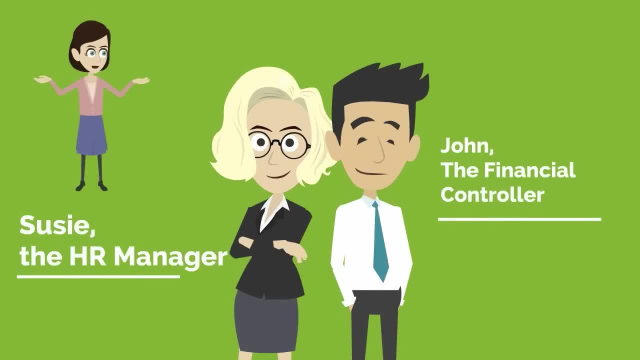 Stakeholders are people or organizations that have some type of impact on our project. For example, Susie from the human resources department can be a stakeholder if we are working on a human resources related system or project. In a similar way, Susie from the human resources department can be a stakeholder if we are working on a human resources related system or project. 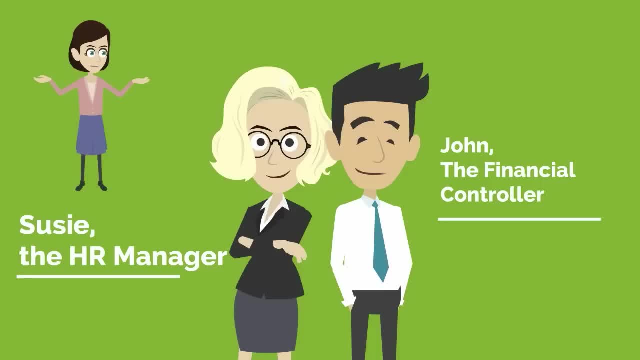 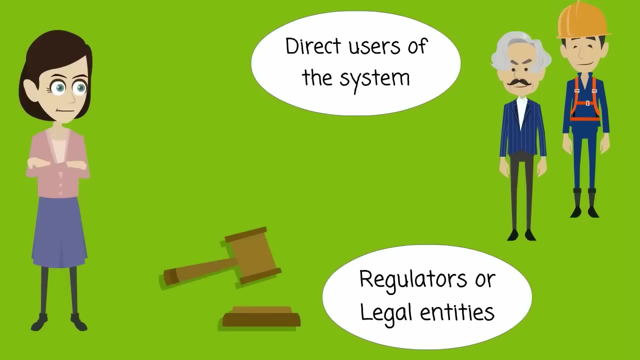 We can have John as a stakeholder if he needs to be consulted about his requirements for the financial aspects, such as a salary and bonus calculation in the context of the human resources system. It is important to identify all the different types of stakeholders early on during your project. 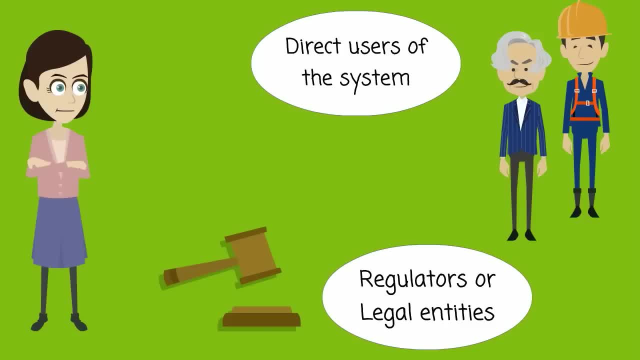 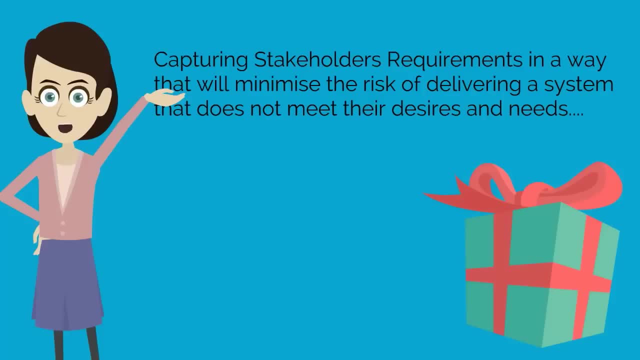 They can be users of the system or their role in the organization could be affected with the implementation of the new system. They can be users of the system or their role in the organization could be affected with the implementation of the new system. then specifying and managing requirements to minimise the risk of delivering a system that does not meet the stakeholders' desires and needs. 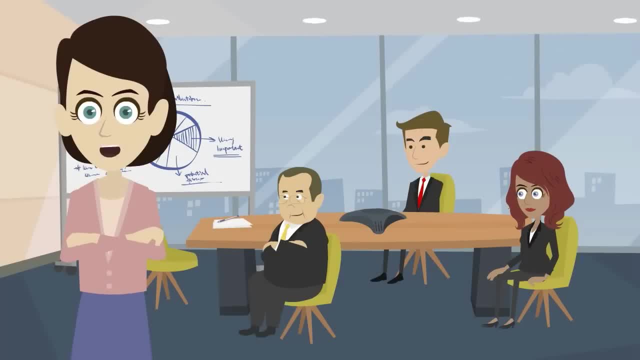 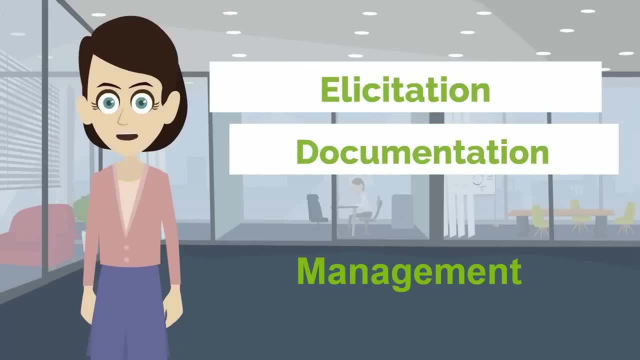 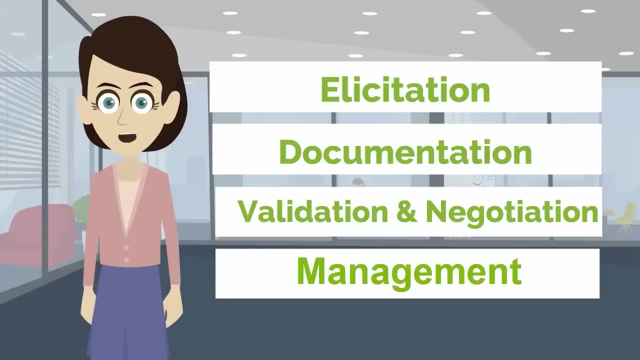 Now that we've covered the fundamental concepts, let's have a look at the four main activities of Requirements Engineering. The four core activities to meet the main goals of Requirements Engineering are as follows: 1. Elicitation, 2. Documentation, 3. Validation and Negotiation, and 4. Management. 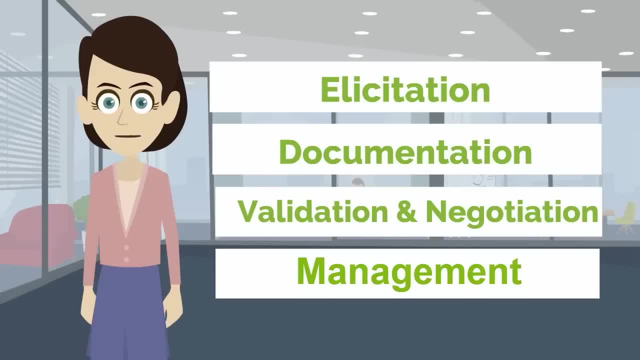 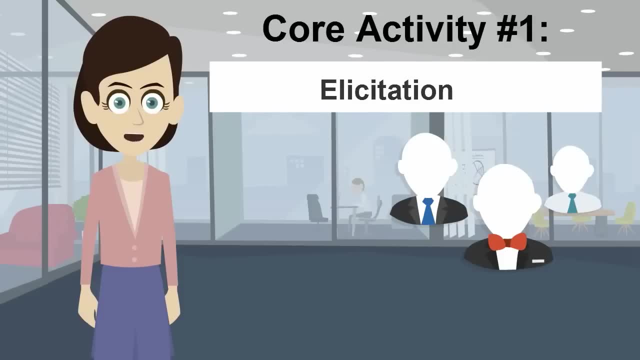 Let's have a closer look at each of these main activities. Core Activity 1. Elicitation. Elicitation is all about engaging with stakeholders to elicit and understand their business needs and requirements. There are various different requirements, elicitation techniques which can be applied. 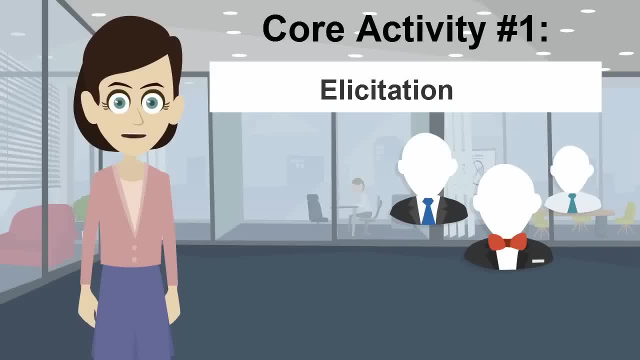 1. Elicitation. Some of these techniques include requirements, interviews and workshops. Core Activity: 2. Documentation: The documentation activity is all about capturing the requirements in a documented format which will make clear sense to the business stakeholders as well as the technical teams who may need your document. 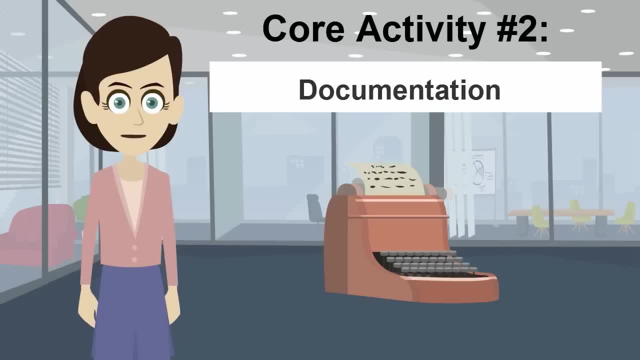 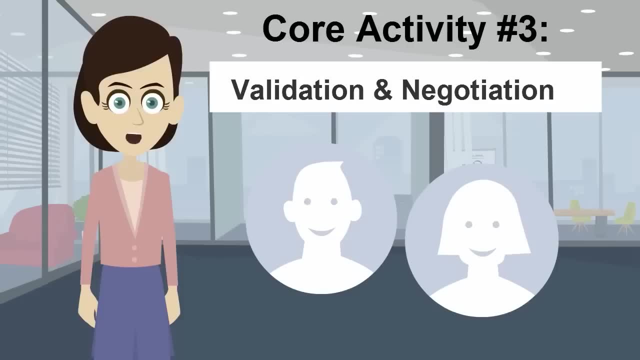 It is important that your requirements are clear, complete and accurate. Core Activity 3. Validation and Negotiation. Core Activity 3. Validation and Negotiation. This activity is all about ensuring that what you have documented as requirements are valid and agreed by all stakeholders involved.